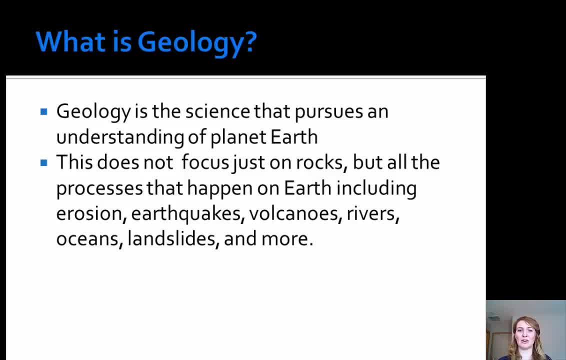 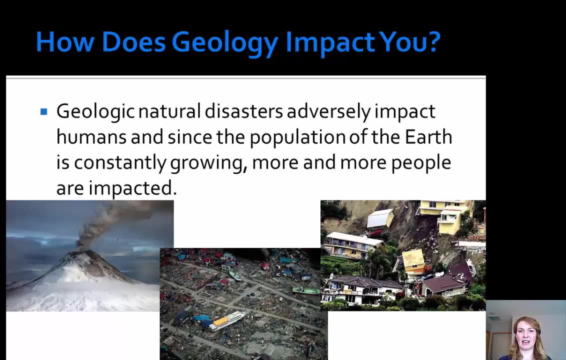 including erosion, earthquakes, volcanoes, rivers, oceans, landslides and so much more. So we're just going to kind of scratch the surface of all these major processes throughout the semester. How does geology impact you? So, geologic, natural. 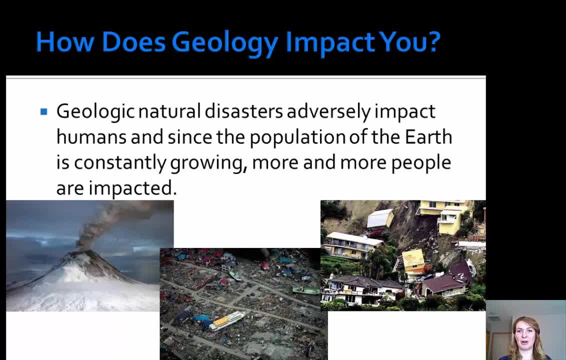 disaster prevention is a major process that we do every year. We do it every year and we do it every year. So geologic natural disaster prevention is a major process that we do every year. So geologic natural disasters adversely impact humans and since the population of Earth is constantly growing more and 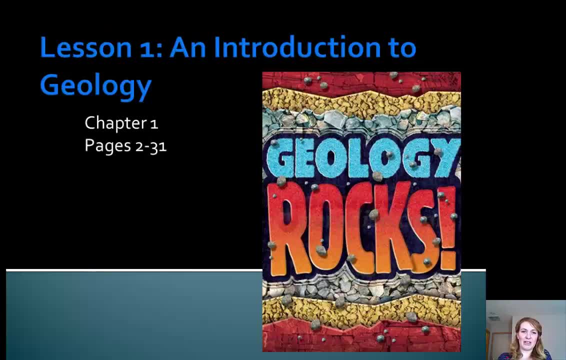 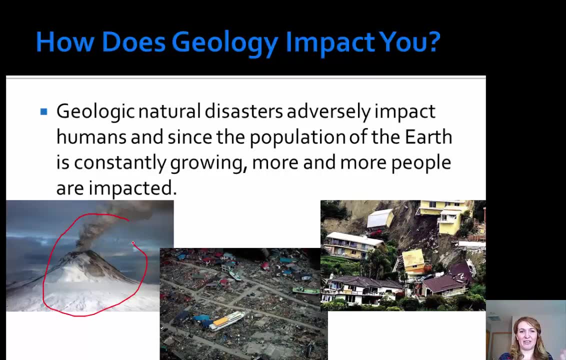 more people are impacted. So right down here, what we All right, so what we have down here, sorry about that. right here we have a volcano and we have a volcanic eruption. that's happening. So we'll talk about how volcanoes and volcanic eruptions impact us. Now, right here, this is going to be the aftermath. 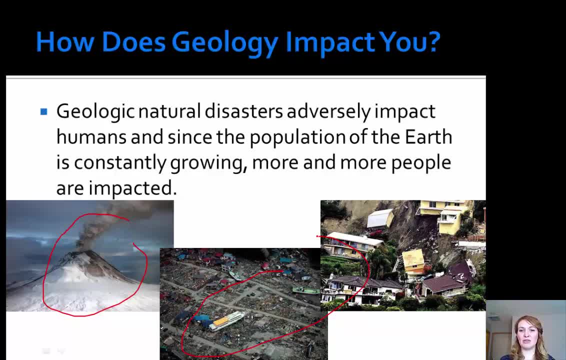 of the tsunami. So we're going to talk about how volcanoes and volcanic eruptions impact us Now, right here. this is going to be the aftermath of the tsunami that was so devastating, And over here, this last photo we see is of a landslide, and we'll talk about the impacts. that landslides and mass 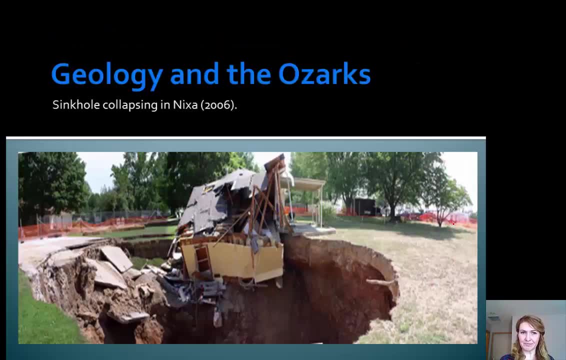 wasting events have on us All right. so just a little bit about geology in the Ozarks and how it adversely affects us. This is a sinkhole collapsing in Nixa back in 2006.. So this is when a gentleman that lived right behind Price Cutter wouldn't have been able to get out of his car. 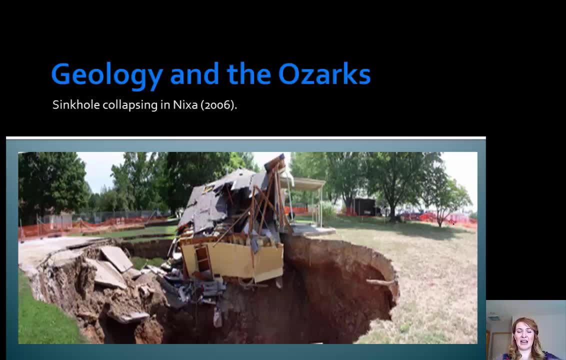 went outside, went to go get in his car and the entire garage pretty much collapsed down into the sinkhole. Now, if you were to go to Nixa today, you would not see the sinkhole. The city has since filled it in. but especially here in the Ozarks sinkholes, karstic systems are definitely something. 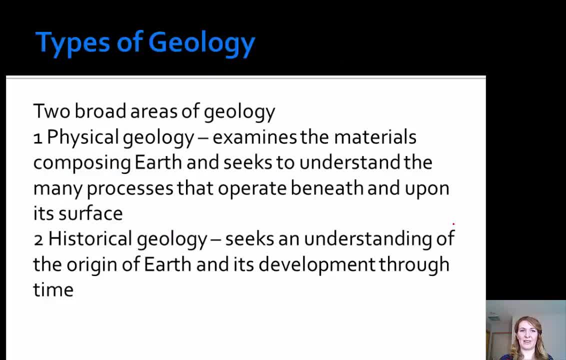 that we have to be concerned about. All right, so we're first going to talk about the different types of geology. So there's really two big broad categories. There's physical geology, and this is going to be where you examine the materials composing earth. 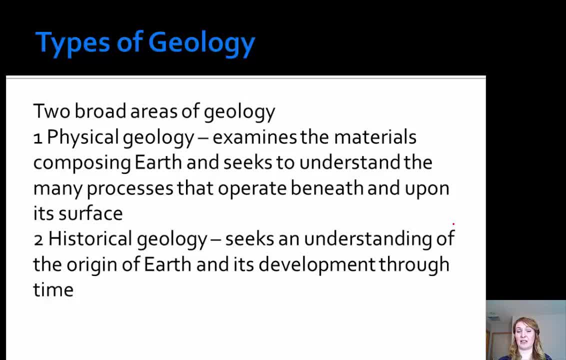 and you seek to understand the processes that operate beneath and upon the surface. So that's mostly what we're going to be focusing on. But the second big area is going to be historical geography, So that's where we're going to try to understand the origin of the earth. 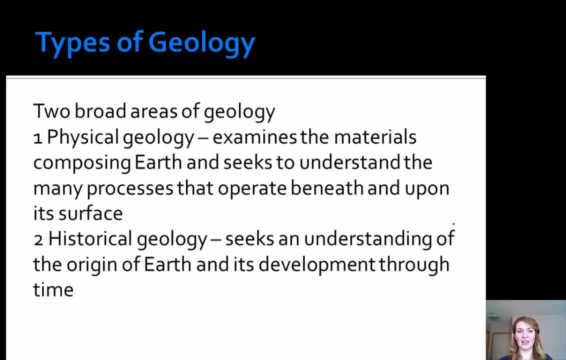 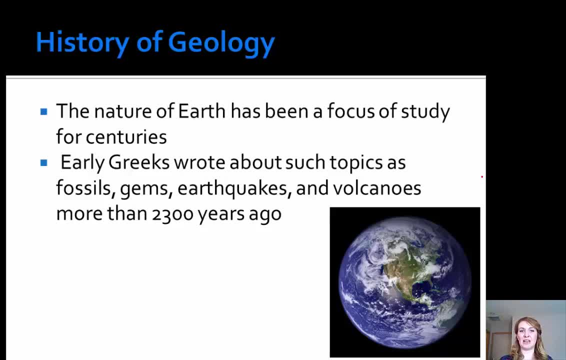 and its development throughout time. All right, so history, geology, So this is pretty basic, and the nature of Earth has been a focus of study for many centuries, So it dates all the way back to the early Greeks, who wrote about such topics as fossils, gems, earthquakes and volcanoes, And so that 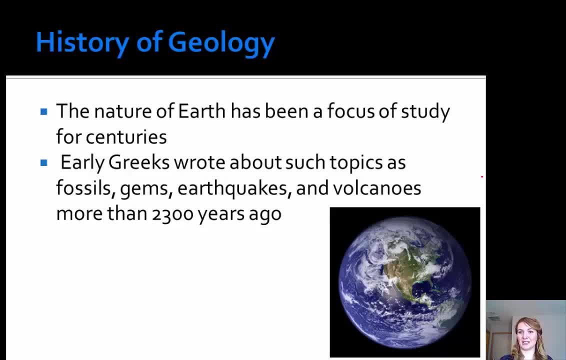 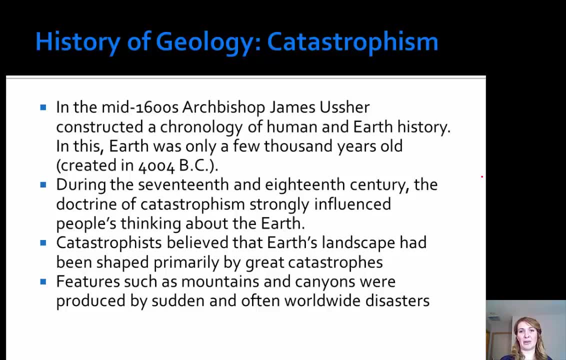 was, more than you know, 2,300 years ago. Alright, so again talking about the history of geology, we're going to talk about catastrophism. So, in about the mid-1600s, Archbishop James Usher constructed a chronology of human and. 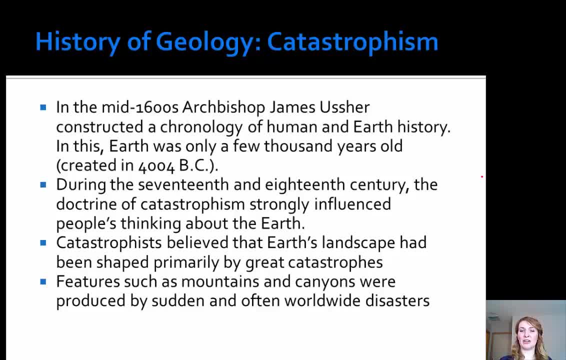 earth history, So in this earth was only about a few thousand years old, created in about 4,004 BC. So during the 17th and 18th century the doctrine of catastrophism strongly influenced people's thinking about Earth. Now these 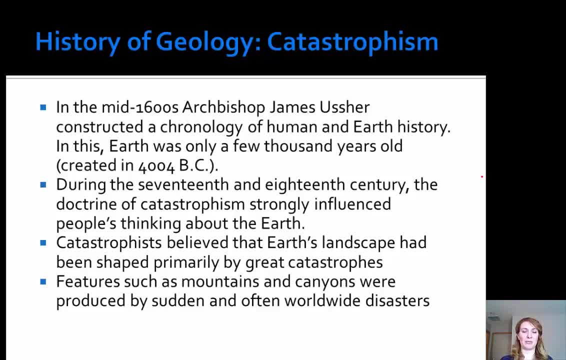 believers thought that the Earth's landscape had been shaped primarily towards the Earth. So they thought that the Earth's landscape had been shaped primarily by great catastrophes. So those are what we kind of talked about earlier. So volcanic eruptions, flooding, tsunamis, landslides, those types of catastrophes. 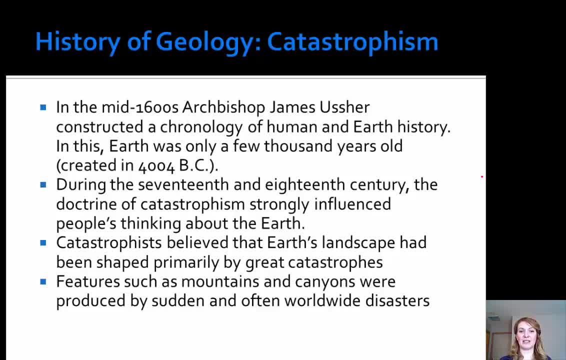 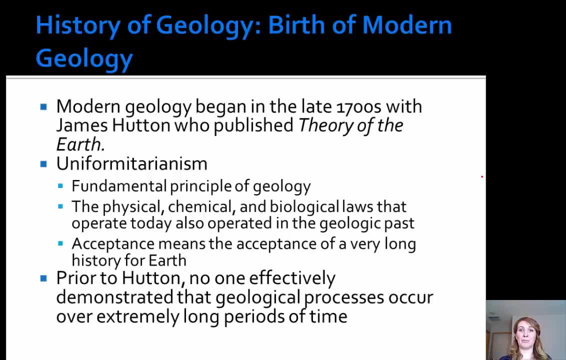 So features such as mountains and canyons were produced by sudden and often worldwide disasters. Alright now, the birth of modern geology began back in the 1700s with James Hutton, who published the theory of Earth. So this is where we introduce the principle of uniformitarism. So this is. 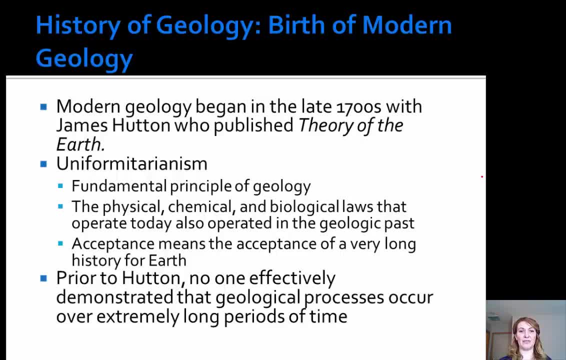 fundamental when we're talking about geology. So the physical, chemical and biologic laws that operate today also operated in our past. So the acceptance of this means that there's an acceptance of a very long history of Earth. So, prior to Hutton, no one effectively demonstrated that geologic processes occur over. 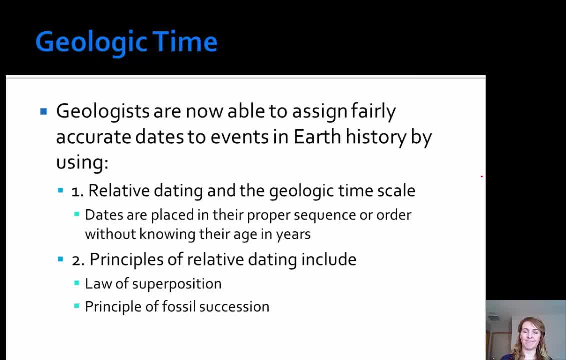 extremely long periods of time. So this is where we introduce the principle of uniformitarism. So this is where we introduce the principle of uniformitarism. So, prior to Hutton, no one effectively demonstrated that geologic processes occur over extremely long periods of time. Alright, now just a quick side note As we go. 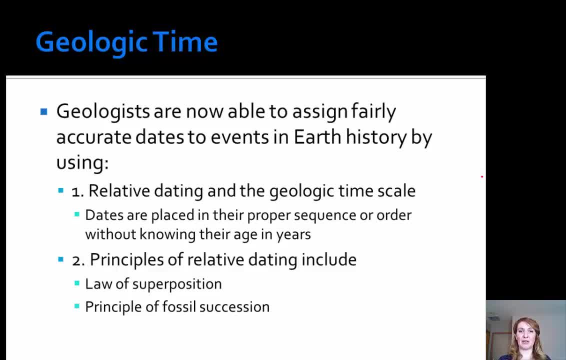 throughout the semester. there's probably going to be some things that we discuss that might challenge some people's religious views, and you might want to talk about those. This class is not the place for that, So we are primarily focusing on geology and the theories that have been presented by scientists over the years. 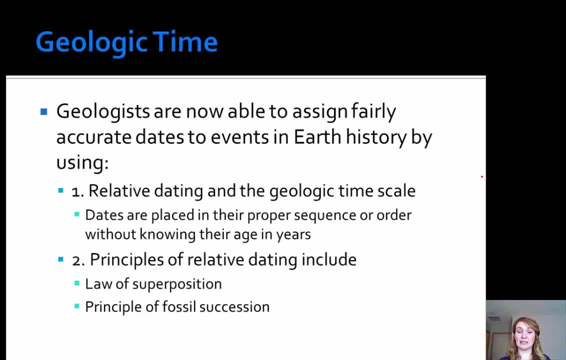 I'm not here to challenge anyone's beliefs, but we're here simply to talk about geology as a science. Alright, so talking a little bit about geologic time. geologists are now able to assign fairly accurate dates to events in the history of Earth by using two 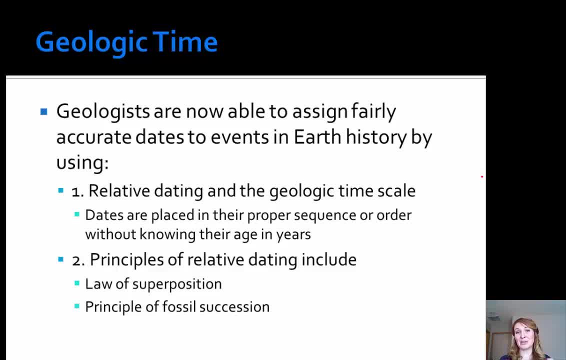 different methods, So we'll talk about this in depth later in the semester, but just to kind of get an idea, the first one is using relative dating and the geologic time scale, timescale, So dates are placed in their proper sequence or order without knowing their age in. 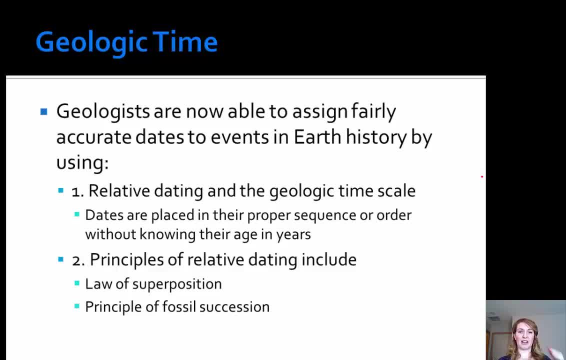 years. So this is saying that. you know we're talking about something that happened first, second and third. So if I were to make a peanut butter and jelly sandwich, first I'd have to get the bread, second, put peanut butter down, third, put jelly down and then put my other piece of. 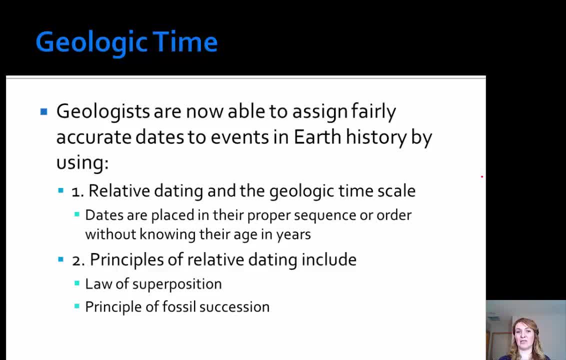 bread down. So that was my relative order of dating how to make a peanut butter and jelly sandwich. Now the second is principles of relative age dating. We're going to be using the law of superposition and the principle of fossil succession, All right, so this is just a very 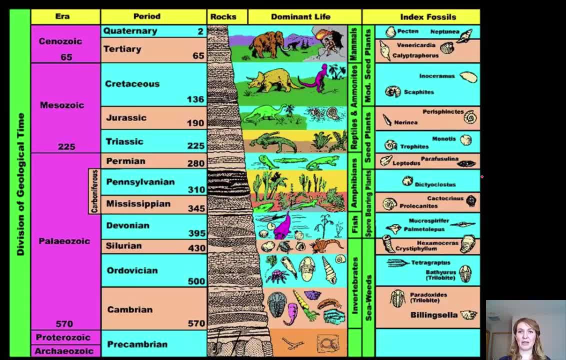 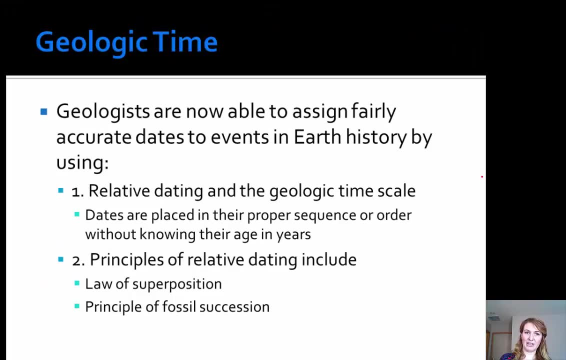 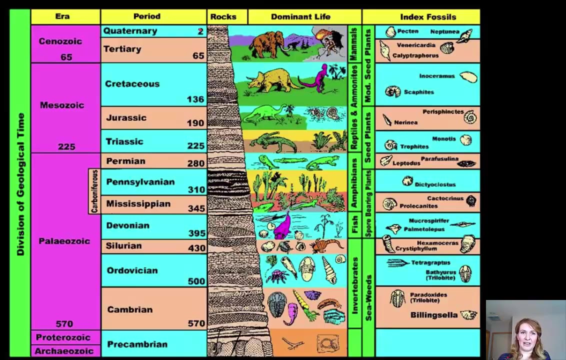 basic idea of the geologic timescale. So it has the eras, the periods, what the racks might look like, The dominant life forms and some index fossils, And so you can see- sorry about that. you can see that the ages here vary all the way from the Cenozoic down to the Precambrian. 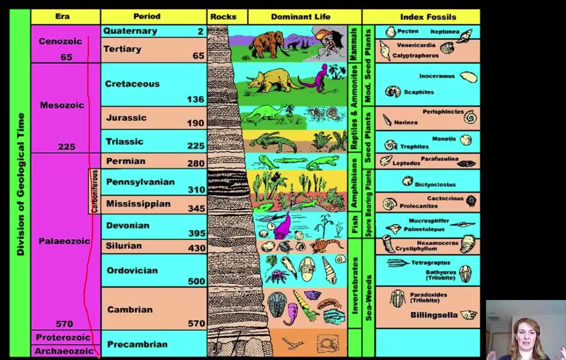 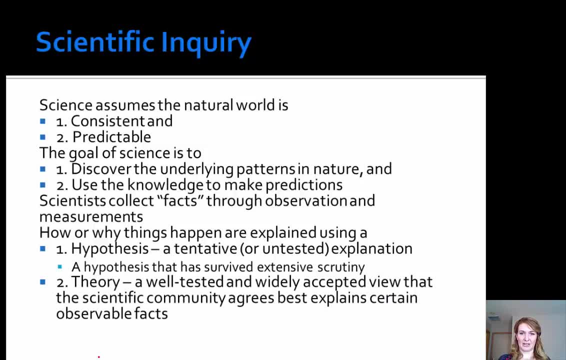 So there's a significant amount of time that is demonstrated on the geologic timescale. All right, so talking about scientific inquiry, So science assumes that the natural world is one that it's consistent and two that it's predictable. Now the goal of science is to one. 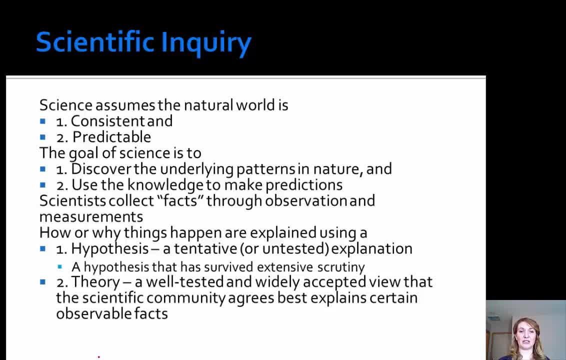 discover the underlying patterns in nature. and two: use the knowledge to make predictions about things that are going to happen in our future. So science assumes that the natural world is one. The hypothesis will collect facts through observation and measurements. So that's what we're going to. 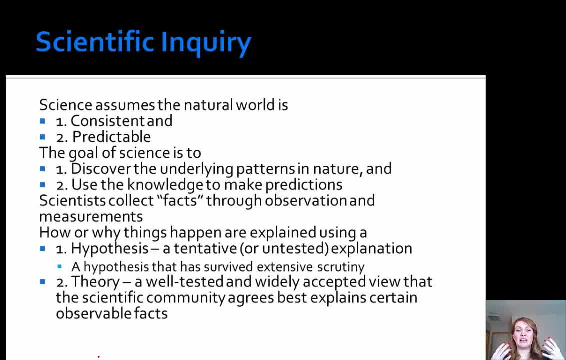 really focus on when we talk about labs, where we're going to be making lots of observations and you're going to also be making measurements. So how or why things happen are explained using first a hypothesis, which is a tentative or an. 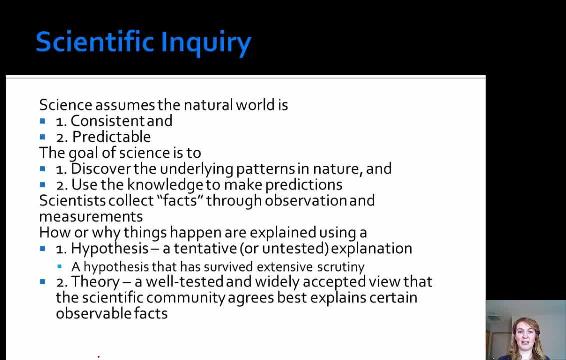 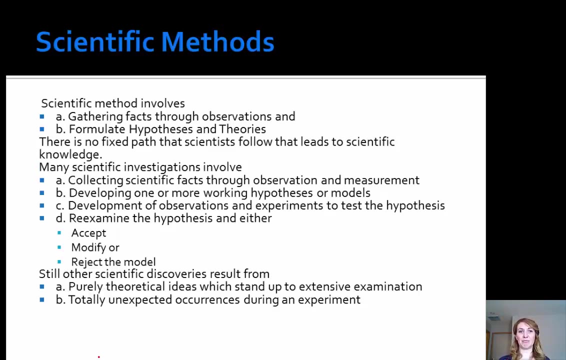 untested explanation. A hypothesis that has survived extreme scrutiny becomes a thing: theory. A theory is a well-tested and widely accepted view that scientific community agrees is the best explanation for certain observable facts. All right, now for scientific methods. we've all talked about this. It's been ingrained in us since we were little, so this is just going. 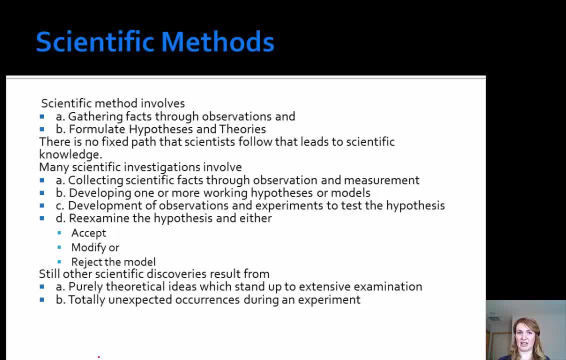 to be a very small overview of scientific methods. So scientific methods include gathering facts through different observations, formulating hypotheses and theories. So there's going to be no fixed path that scientists follow that leads to scientific knowledge. So if I were to approach a subject such as you know why gold forms and 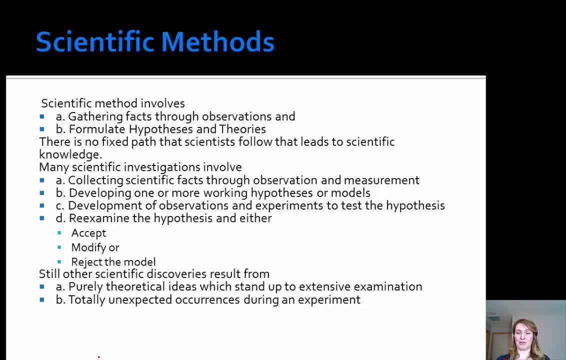 one location and not in other. I might go through steps A, B, C and D. Now if my colleague, whoever it is, approaches the same subject matter instead of going through A, B, C, D and E, 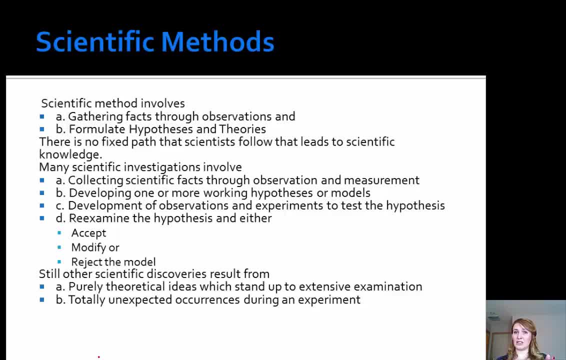 they might do A, D, F and G, So we never have to follow a fixed path. Scientists take very different paths and most of the time we reach the same goals. All right, so many scientific investigations will include collecting scientific facts through observation and measurement. 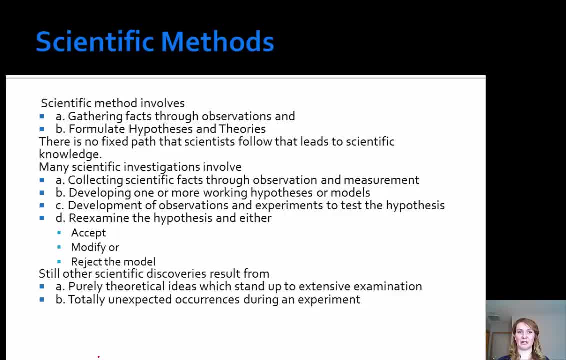 developing one or more working hypotheses or models, development of observation and experiments to test the hypotheses or models. then you're going to re-examine that hypothesis or either, based on that, you're going to accept it, modify it or reject it. Now, still other scientific discoveries result from purely 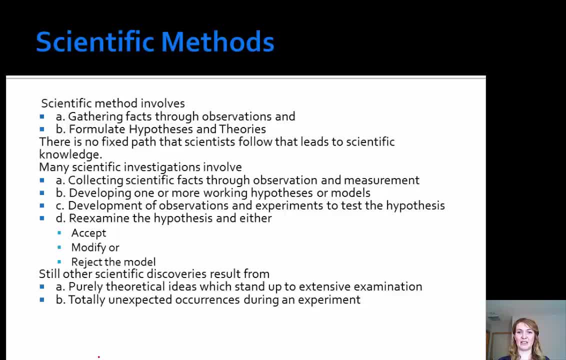 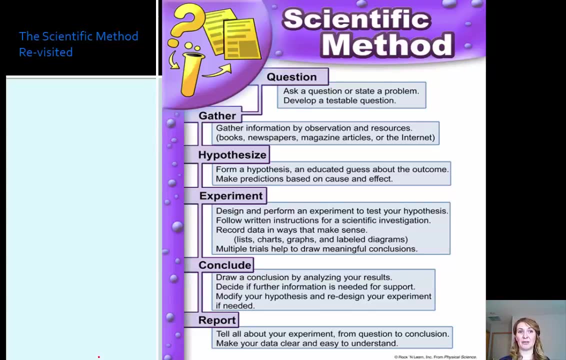 theoretical ideas which stand up to extensive examination or totally unexpected occurrences during an experiment. All right, so again, this is going to be the scientific method that's revisited. So you question, Question, you gather, hypothesize, experiment, conclude and report. 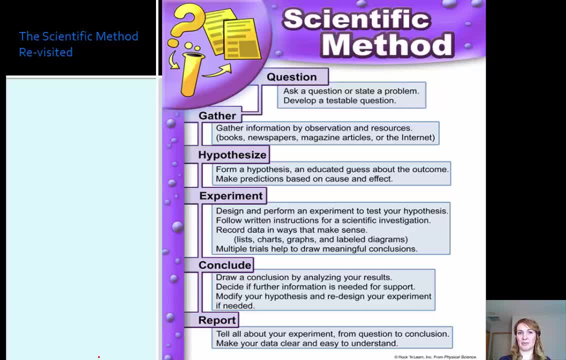 So this is going to be an important foundation for us all to remember as we go throughout the semester. There will be several times where I ask you to hypothesize what some observations and measurements could mean. Now, when I ask you to do that, we're going to be doing an educated guess based on the outcome. 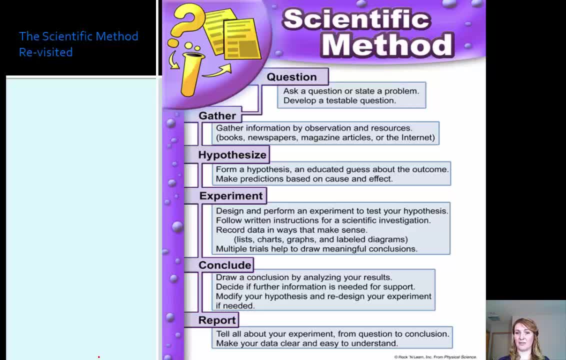 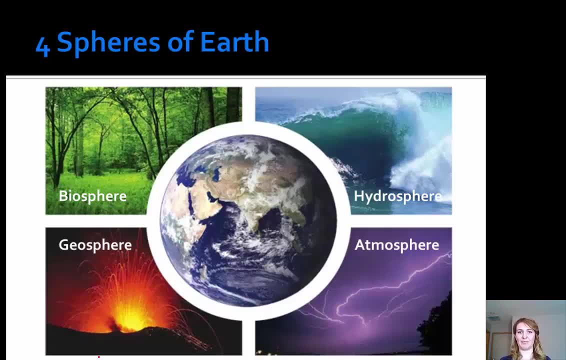 We're going to make predictions based on cause and effect. All right, so we're going to move on to what the four spheres of the Earth are. So there's four spheres: We have the biosphere, hydrosphere, geosphere and the atmosphere. 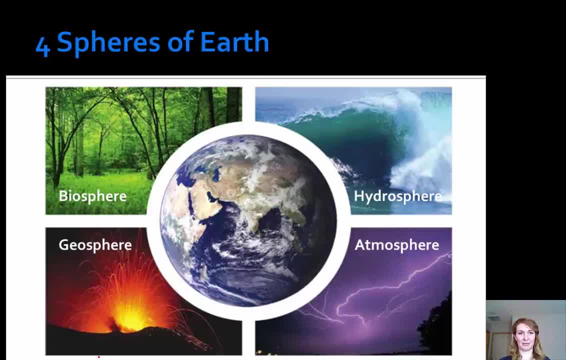 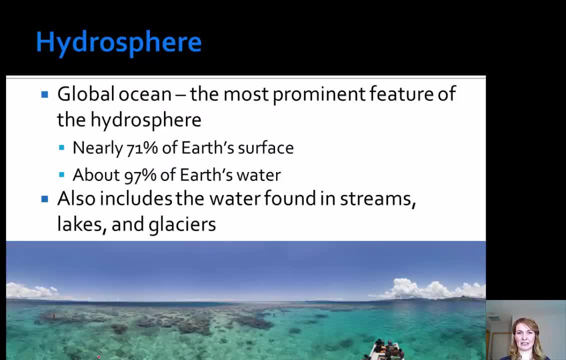 So we're going to talk about each one of these in a little bit more depth. So the hydrosphere. So hydro meaning water, So this is the global ocean, So the most prominent feature of the hydrosphere. So nearly 71% of the Earth's surface is contained in the hydrosphere. 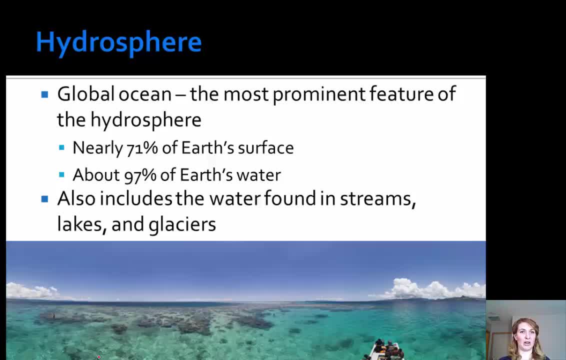 And about 97% of all of Earth's water is based in the hydrosphere, So this also includes water found in streams, lakes and glaciers. So on the image down below, you can see this massive, beautiful view of all the water. So that is the hydrosphere here. 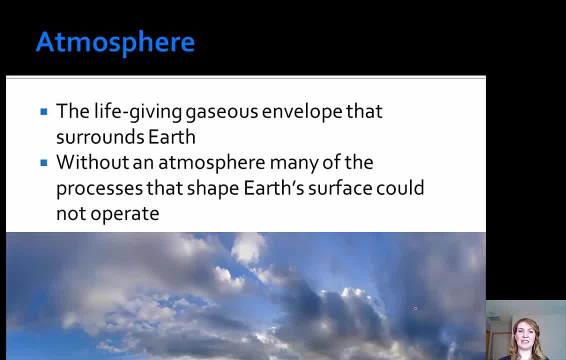 All right. so next is the atmosphere. This is the life-giving gaseous envelope that surrounds the Earth. So without an atmosphere, many of the processes that shape the Earth's surface wouldn't be able to operate. So we're talking about wind, which produces erosion, different things like that. 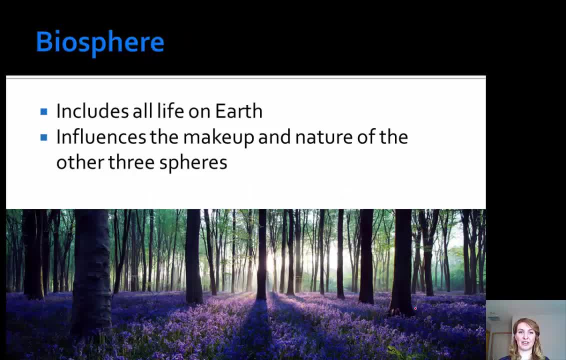 All right. So the biosphere? This includes all life on Earth, even us, and it influences the makeup and nature of the other three spheres. So in the image below, it's pretty easy to see what the biosphere is. We have trees that are growing up. 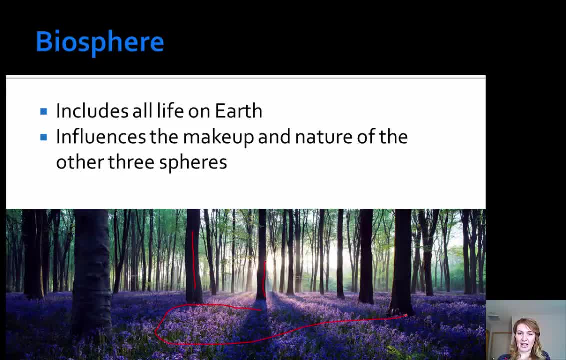 We also have these flowers down through here, And you can see a lot of different greenery in all of the image, So some of it's related to trees, Some of it might be related to something else, But that's what's making up the biosphere in this image. 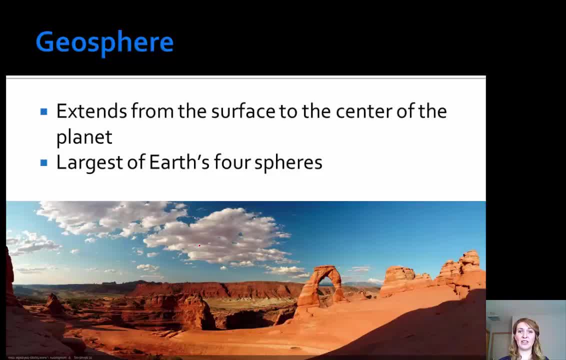 All right. So the geosphere: this extends from the surface of the Earth down to the center of the planet. So this is the largest of all four spheres. So geo- think about rocks and stuff like that. So when we're looking at this image, we see this beautiful arch here made up of rock. 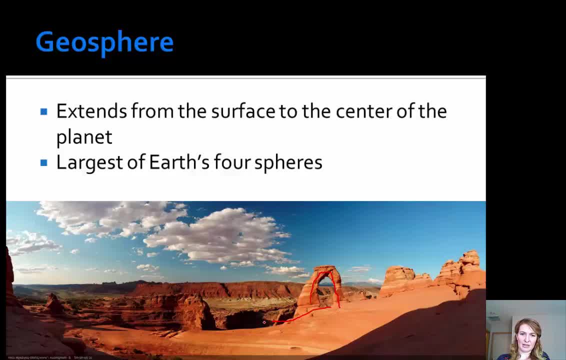 That would be part of the geosphere, Same with all of these rocks down through here. We have the canyon right over in here. All of that is part of the geosphere. Now, up here, what we're looking at, this is going to be the atmosphere. 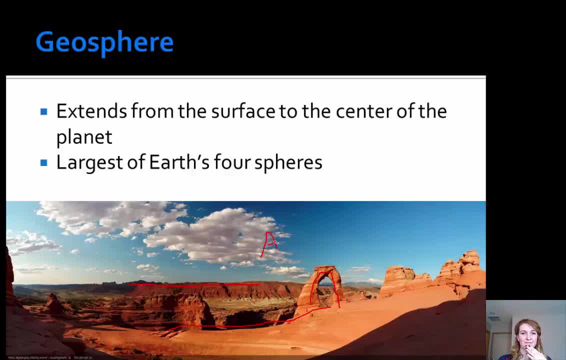 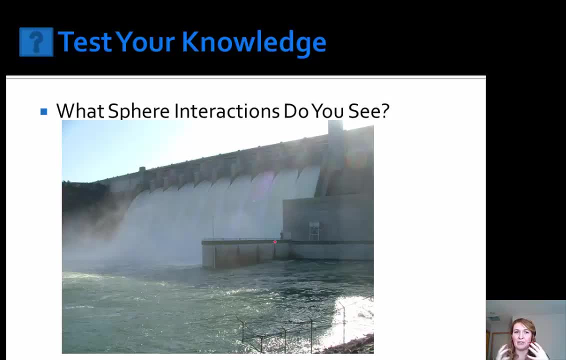 That's the envelope that surrounds the Earth. All right, So we're going to test our knowledge. So what sphere interactions do you see? First, we need to identify what spheres we even see, right? So remember, we have the biosphere, hydrosphere, atmosphere and the geosphere. 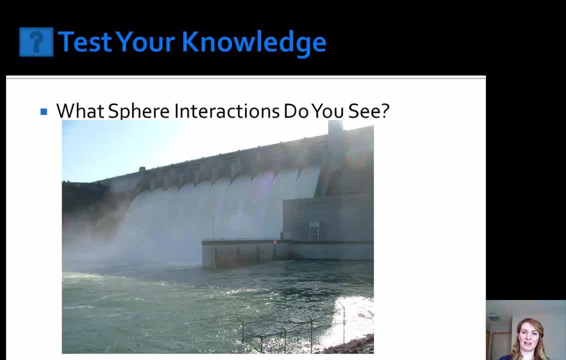 So this is a dam that's down at Table Rock Lake. Now, first off, I see the hydrosphere. That's all the water that's down here. Now, when I look up above the dam in this area, I see sky. 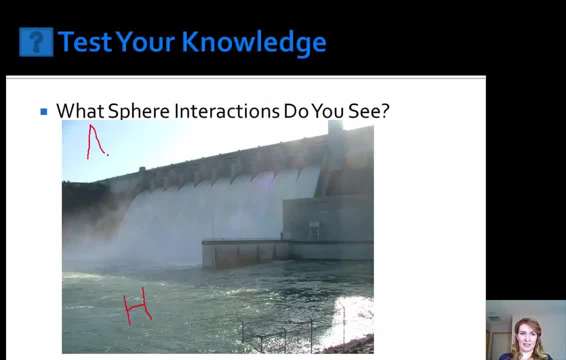 That is going to be part of the atmosphere, So I'm going to put an A Up here for atmosphere. Now, this is a man-made structure. This is not a natural dam, So this is how humans have been introduced into this. 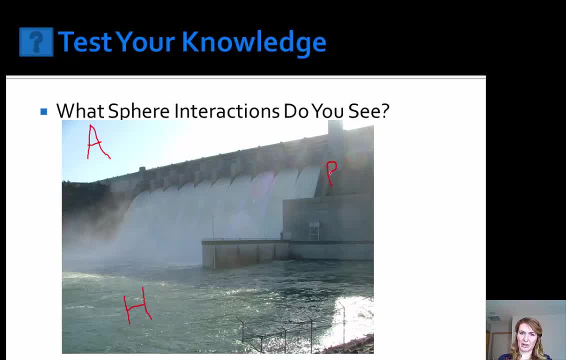 So that is, creating. that is part of the biosphere here. But in addition to it being a biosphere, we're going to add a little plus sign. This is also made up of geosphere materials. So I'm not sure, We're not sure- exactly what the material is that's making up the dam. 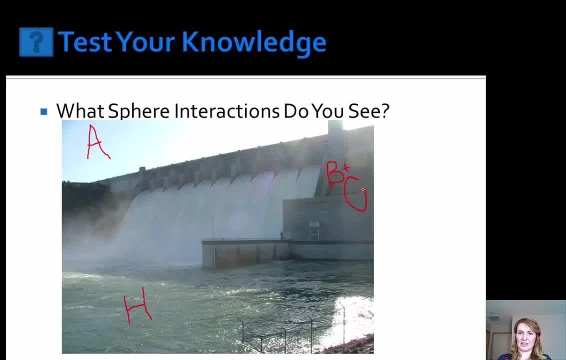 But we know that's going to be related to the geosphere. Alright, so those are what spheres we see. So let's think about how they're all interacting together. How is the water related to the atmosphere, Related to the biosphere? 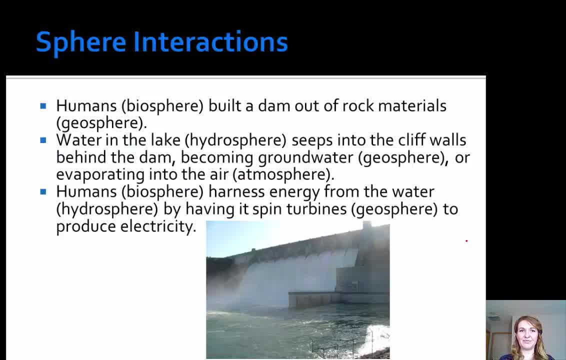 Related to the geosphere. Alright, so this is how we're going to break it down: Humans, Humans, the biosphere- built the dam out of rock materials, which is our geosphere. Water in the lake hydrosphere seeps into the cliff wall behind the dam, becoming groundwater geosphere. 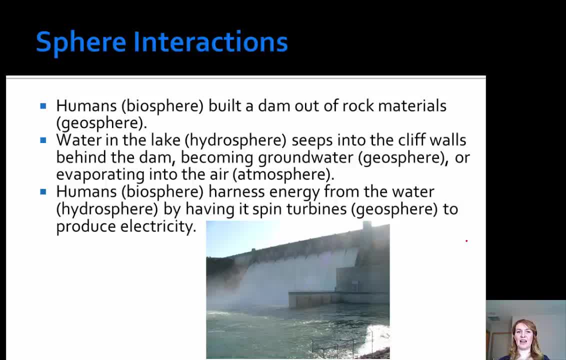 Or evaporating into the air, which is the atmosphere. Humans which make up again the biosphere. harness the energy from the water, hydrosphere by having it spin turbines, geosphere To produce electricity. So you can see how something as simple as a dam incorporates all the different spheres. 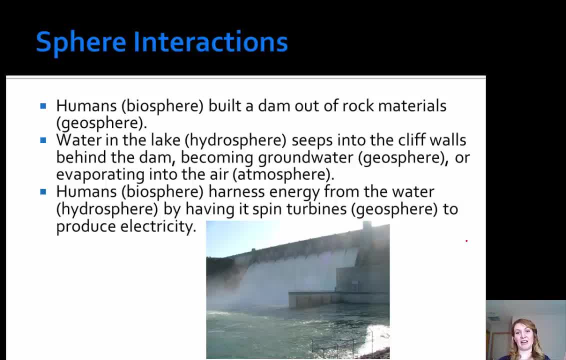 And they're all interacting together. Now I encourage you to do this sort of critical thinking activity on your own, with just different images that you see. Try to relate the biosphere, the geosphere, hydrosphere and atmosphere all into one thing. 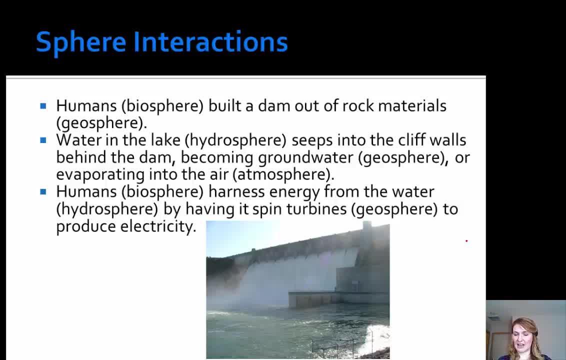 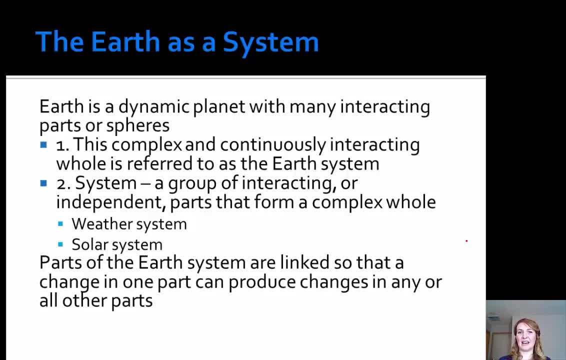 See how each little thing Is impacting everything else. Alright, so talking about that, Earth can be seen as a system. So Earth is a dynamic planet with many interacting parts or spheres, So this is complex and it's continuously interacting as a whole. 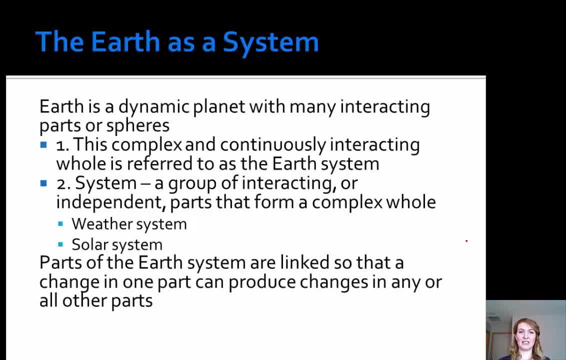 So that's referred to as the Earth system. Now the system is a group of interacting or independent parts that form a complex system. Now the system is a group of interacting or independent parts that form a complex system. Now, the system is a group of interacting or independent parts that form a complex system. 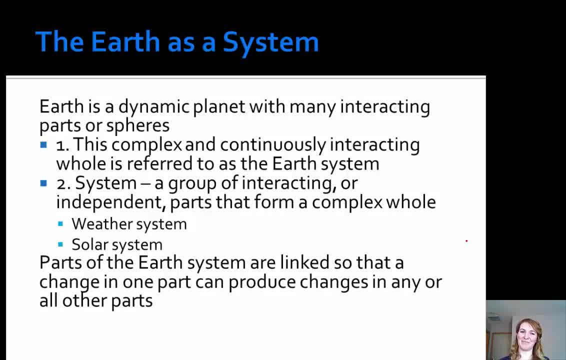 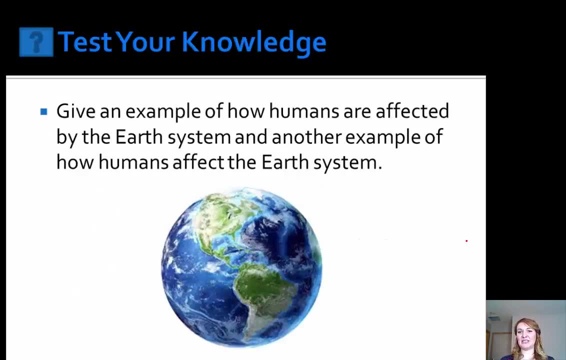 So we have a weather system, we have a solar system, different things like that. So parts of the earth system are linked so that a change in a part can produce changes in any other part or all other parts as a whole. Alright, so we're going to do another little test your knowledge question. 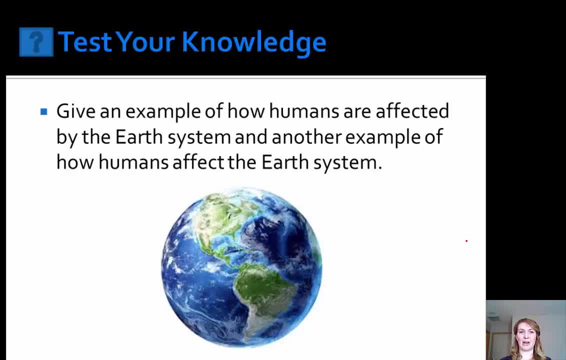 So give an example of how humans are affected by the earth system And another example of how humans are affected by the ecosystem And another example of how humans are affected by the ecosystem, affect the earth system. I'll give you a couple minutes to kind of think of something. The first: 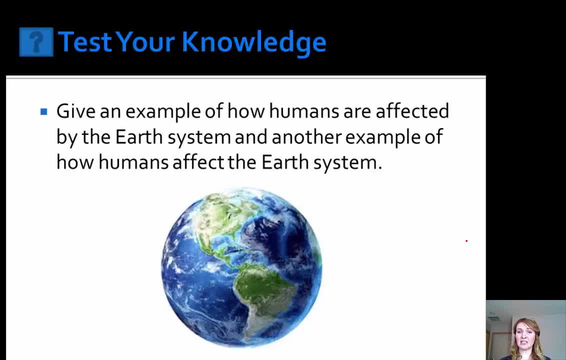 thing that comes to mind with how humans are affected by the earth system are those natural disasters we talked about earlier. So when we talk about volcanoes, earthquakes, tsunamis, landslides, flooding, sinkholes, those are all related to how humans are affected by earth system. 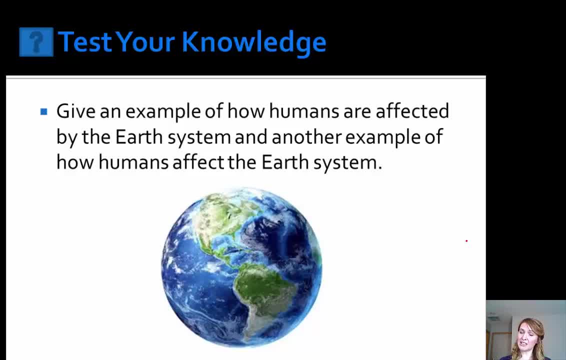 Now another example of how humans affect the earth system. let's go back to that dam example. We build dams, we also have windmills, we harness energy, but all of those are affecting the earth as a system, but the earth system affects us individually as well. 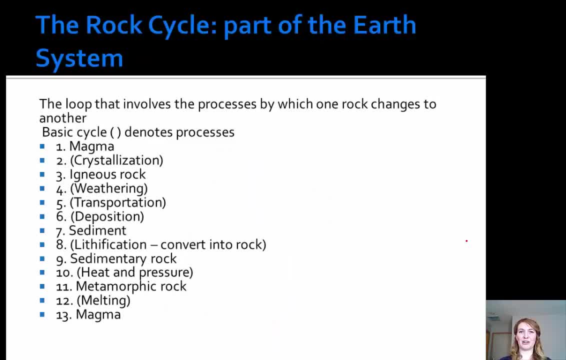 All right. so moving on To the rock cycle, a part of the earth system. So this, the rock cycle, is a loop that involves the processes by which one rock will change into another. So we'll talk about all of these more detail as we go throughout the semester. So the parentheses are going to denote processes. 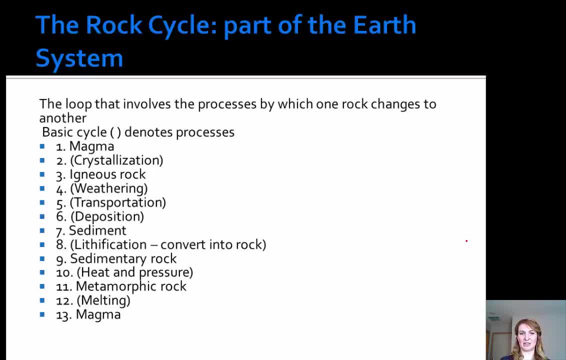 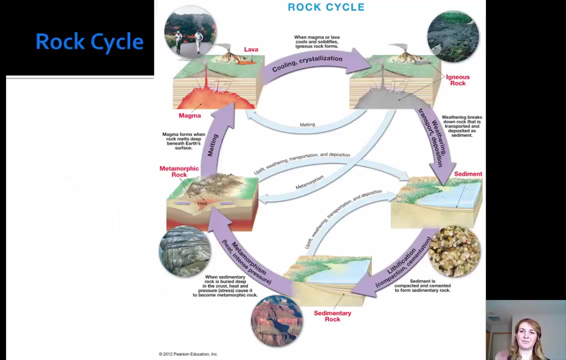 So we have magma, crystallization, igneous rocks, weathering, transportation, deposition, sediment lithification, which is converting something into a rock, sedimentary rocks, heat and pressure, metamorphic rock, magma and melting, All right. so let's take a look at the rock cycle. So we have an image of it right here. 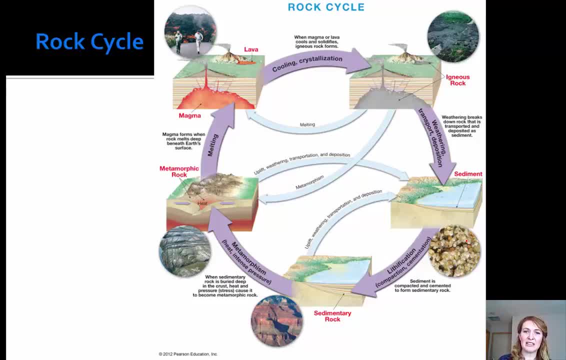 So we can see. you know, this is a complete cycle and there's not one path to reach any one thing. So you know, going to, let's say, metamorphic rocks, So we have several different paths If you follow this area from. 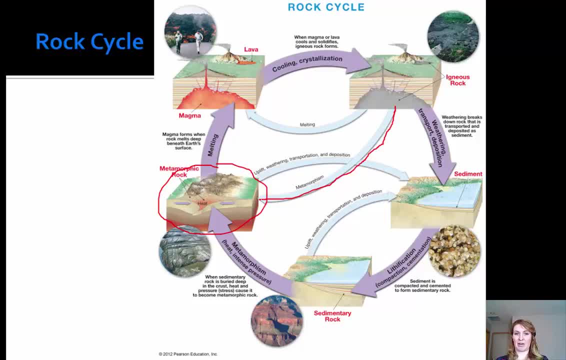 igneous rocks, we can have metamorphism and we have metamorphic rocks, But we also can get there from sedimentary rocks down here. So we have metamorphism with heat and intense pressure. So there's several different ways to get to any one part of the rock cycle. So there are 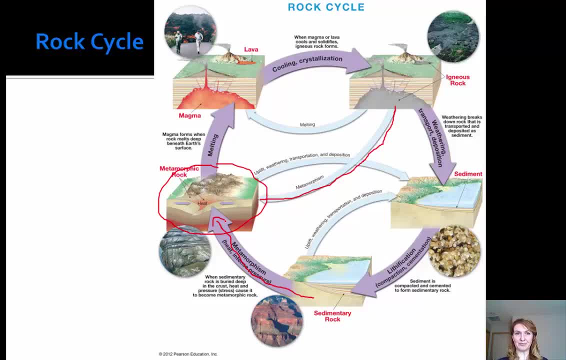 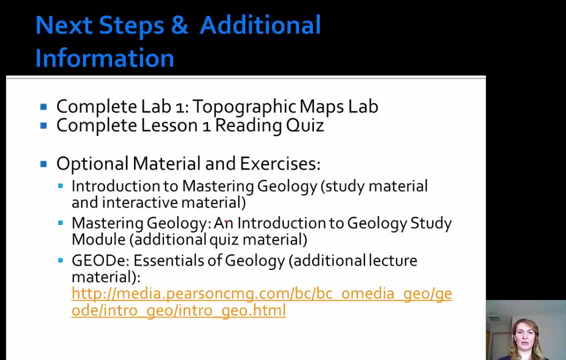 two different ways to get to any one part of the rock cycle, and they are all interacting and connecting to one another. All right, so just talking about next steps and additional information. So what you need to do now is complete Lab 1,, which is based off of topographic maps. 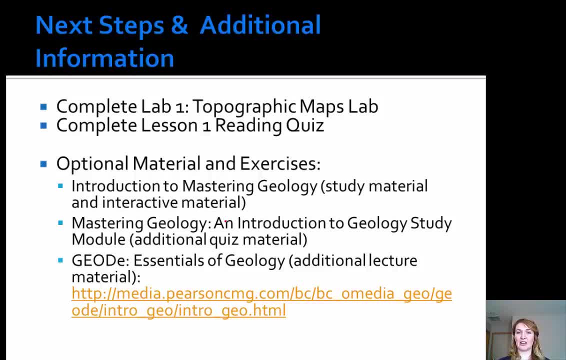 You're going to complete lesson one reading quiz, So this is a ten question quiz that goes over material not only covered in the lesson that I presented, but also textbook information: 10 questions, birth, 10 points, unlimited times that you can take it, and there's no time. 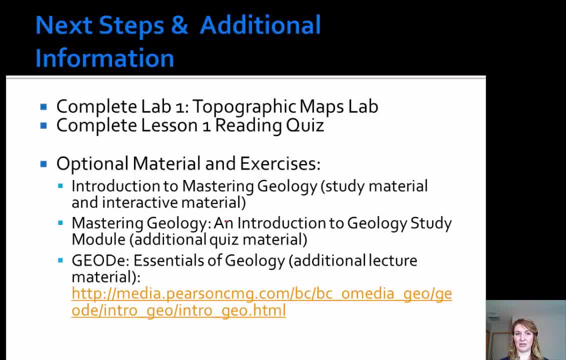 constraint on it. Just have it turned in by the due date. Now some optional material and exercises you can do an introduction to mastering geology. There's study material and interactive material Mastering geology. there's an introduction to geology study module. so that's additional quiz. 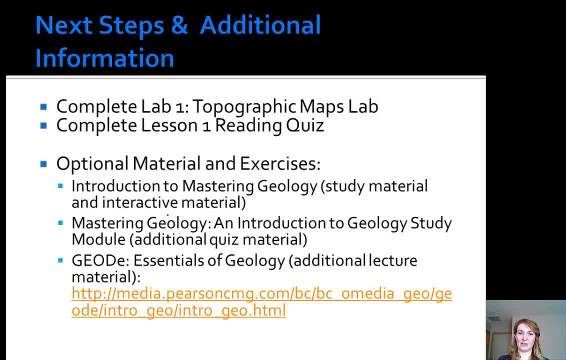 material and you can also click on this geode link down here. So let me just change out of this so that I have my arrow. So if I click on this, this is going to take me to a website. Maybe Give it a minute.